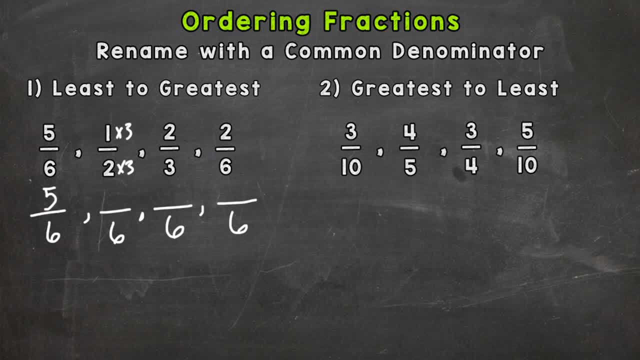 In order to rename that fraction. So one times three is three. Three times two gives me the denominator of six, So I need to do the same thing to the top in order to rename that fraction. So two times. Oh, I'm sorry, I did three times two, So I need to do two times two would give me. 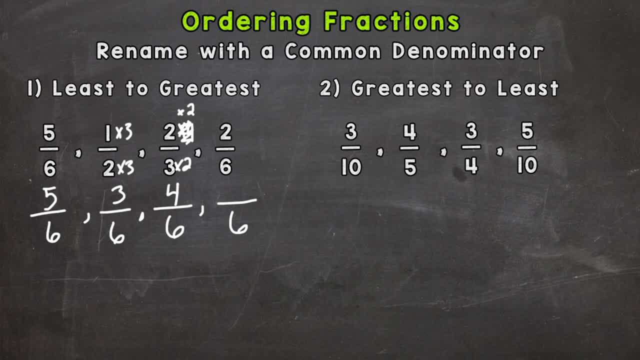 four, And then the last one, Two-sixths is already out of six. Two-sixths is two-sixths. You do not need to rename Now. that makes it much easier to order these fractions because everything has the same denominator. So, least to greatest, our least is going to be two out of six, right, Two-sixths. 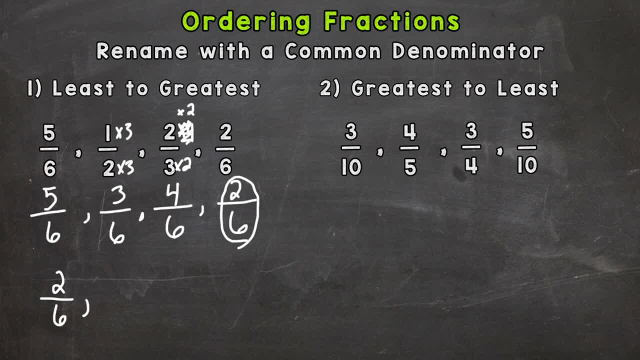 Next. well, we have a five-three-and-a-half And a four. obviously are three-sixths here or one-half. I'm going to put the original fraction in my order down here at the bottom. Next would be four-sixths or two-thirds from the original list. 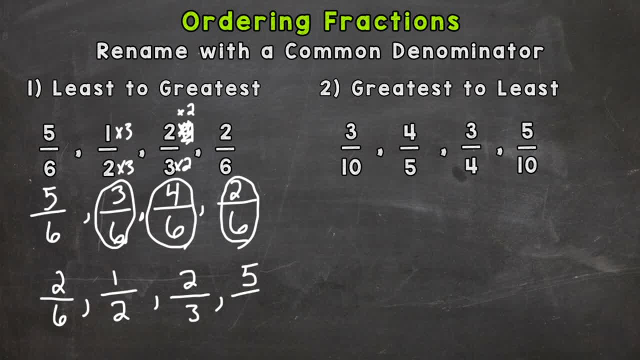 And then, lastly, the greatest fraction, five-sixths. And there you have it. Those fractions are now in order From least to greatest. This is the final answer here, So let's go to number two, where we're going to go greatest to least. 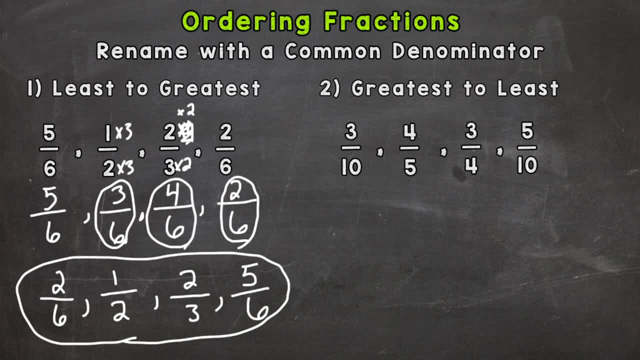 But it's the same process: Find a common denominator, rename and then put them in order. So here we have three-tenths, four-fifths, three-fourths and five-tenths. So we need a common denominator for all four of those fractions. 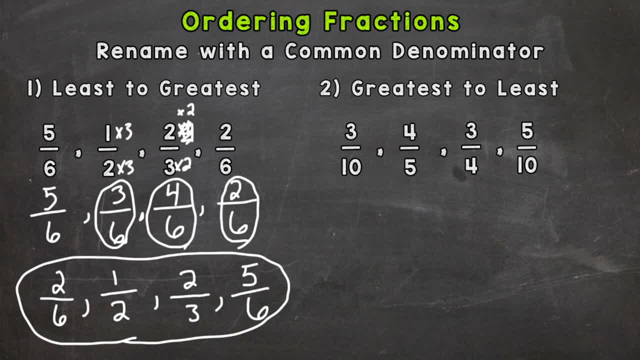 So we have a ten, Five, four and ten. Any idea what the common denominator is for those fractions? Hopefully you're thinking twenty, So let's rename with the denominator of twenty. All right, Well, three-tenths, we need to see how do we get ten to equal twenty and then do that. 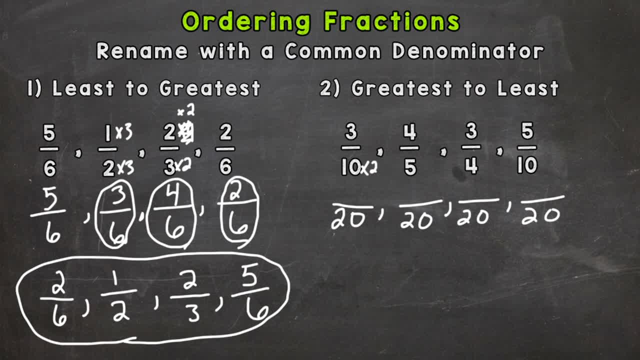 to the top as well. Well, I know, Two is twenty, So three times two is six, So three-tenths is equivalent to six-twentieths. I'm not changing the problem or the value of these fractions when I rename. 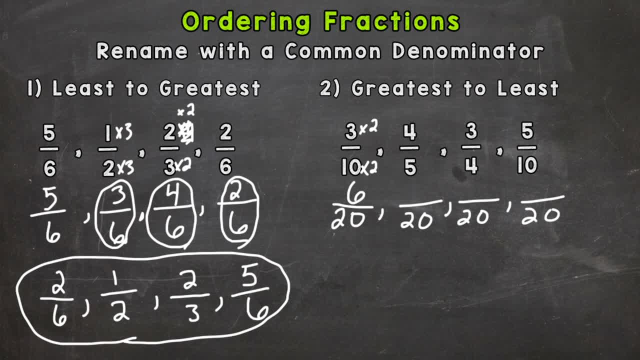 I'm just finding equivalent fractions with a common denominator, All right. Next, I know five times four is twenty, so I need to do the same thing to the top: Four times four is sixteen. Next, I know four times five will give me that denominator of twenty. 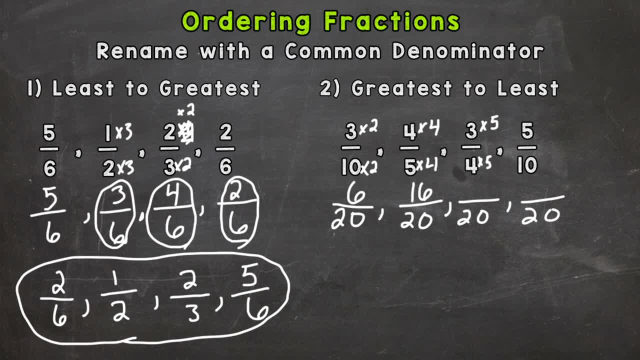 So I need to do the same thing to the top. Three times five is fifteen. And lastly, ten times two is twenty. Five times two is ten. Now that everything's out of twenty, it's much easier to put these in order. 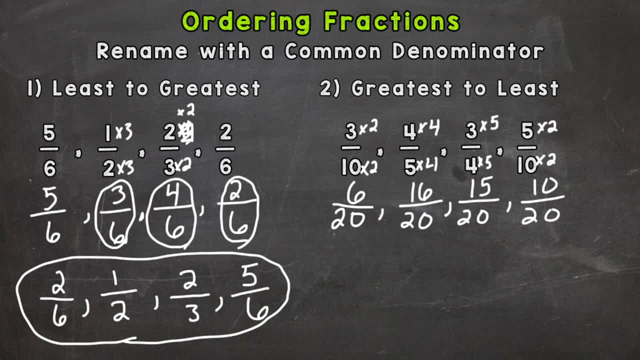 So we need the greatest first. So we have sixty, Six-twentieths, sixteen-twentieths, fifteen and ten. Well, sixteen-twentieths is the greatest, And I'm going to put the original fraction first. four-fifths: 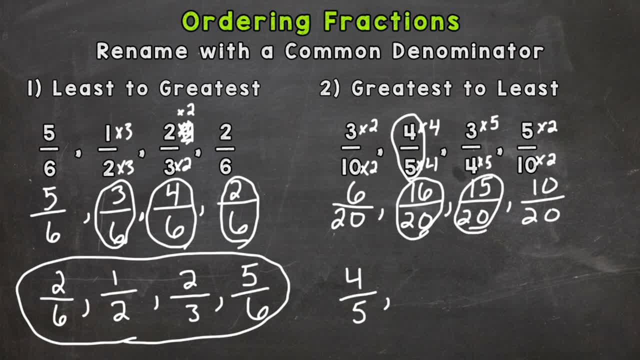 Next would be fifteen-twentieths, And the original fraction is three-fourths, Then ten-twentieths, which is five-tenths, Ten-tenths in the original list, And lastly six-twentieths, which is three-tenths in the original list. 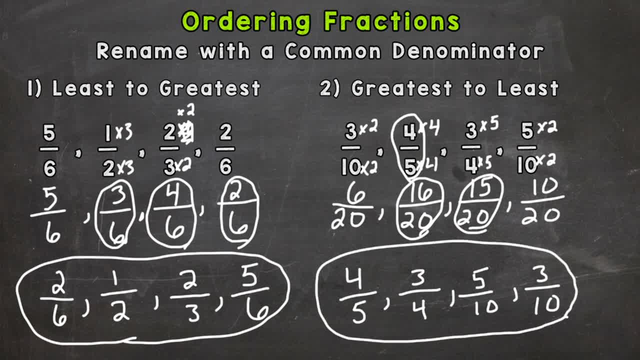 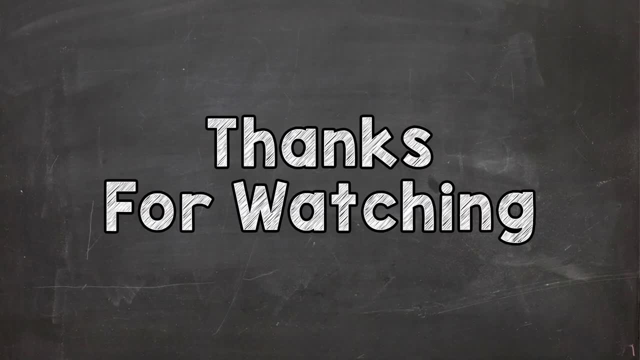 And there's our order from greatest to least. So there you have it. There's how you order fractions. Find that common denominator, rename the fractions using that common denominator and then it's easy to put those fractions in order. Thanks so much for watching. Until next time, peace, Bye-bye. for some to explain the difference between value sales, unit sales and volume sales with respect to the fmcg industry. let's get a bit technical for a minute and go over a simple example. brand ola sells a 500 milliliter bottle of orange juice which the consumer buys at the